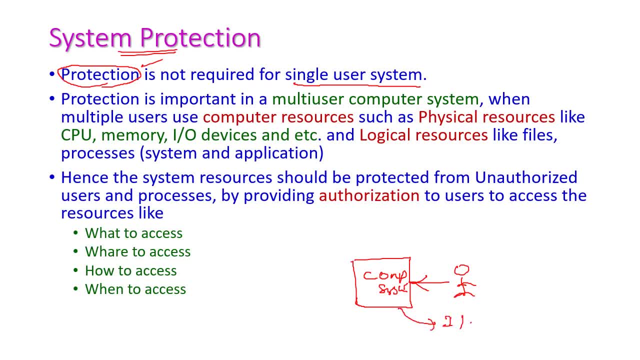 But if the system is connected to internet or if it is a multi-user computer system, then the protection is very important. right See, when multi-user computer system, the computer resources should be protected What type of resources we are having. We are having both physical resources and logical resources. Physical resources are nothing but the CPU, memory, I-O devices, and logical resources are the files and processes. 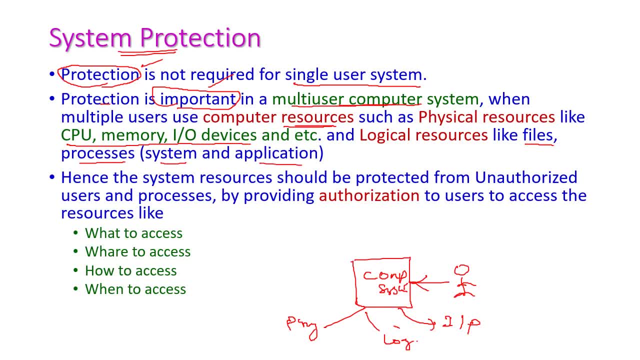 That may be the system programs and application programs. Everything will come under logic. So we have to protect both physical resources as well as logical resources from malicious users or malicious programs. Hence the system resources should be protected from unauthorized users and unauthorized processes. 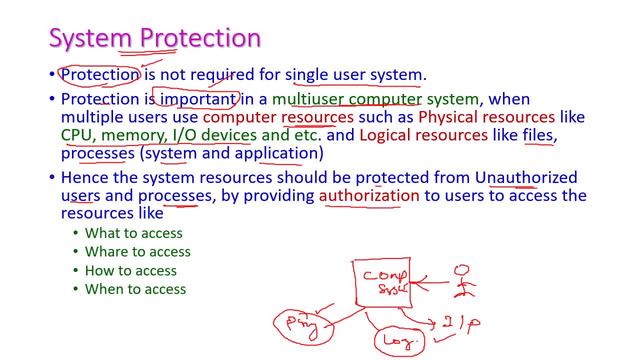 How we can prevent those access By providing the authorization to the users to access the resources. See what are the authorizations We can provide. what to access, That is, which resources are the user being allowed to access? Second, one is where to access, In which place the user have to access those resources, and how to access and when to access. 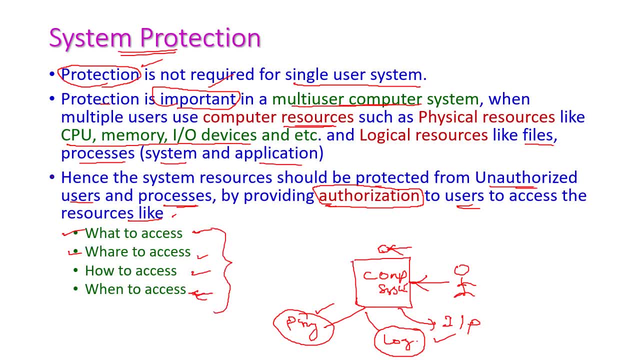 That is the time limit. So the user should follow these conditions. Then only we can protect our system from the unauthorized users. So what to access, where to access, how to access and when to access- These are very important in the system protection. 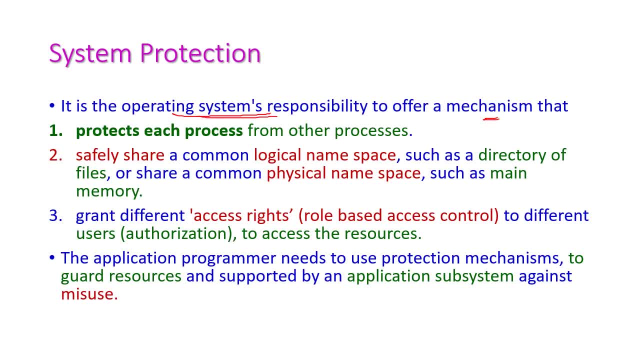 It is the operating system's responsibility to offer mechanism that protect each process in the computer system from external processes. We have to protect each and every process of our computer system And the second important one is safely share the common logical namespace. The common logical namespace means the directories and files. 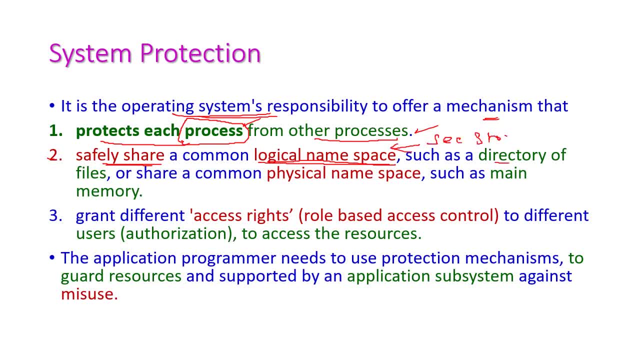 That is the secondary storage. Secondary storage files are the physical namespace That is the main memory. So safely share the logical namespace as well as the physical namespace. And third important one is access rights: To provide access rights to all the users. 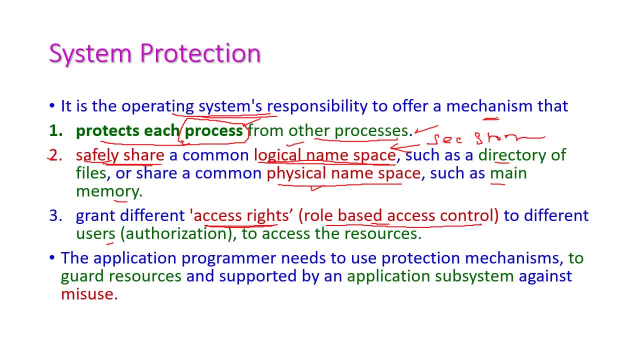 That is, role based access control to different users, That is, by providing authorization to access the resources. This is the third important one. Hence the application programmer needs to use protection mechanism. The application programmer have to implement all these mechanisms to guard the resources. 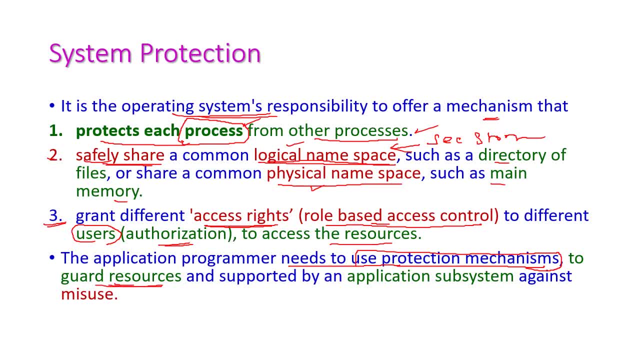 To guard the system, resources and support by application subsystem against misuse. This is called as protection And these are actually the goals of protection. So we have to protect each and every process and the memory, as well as the other resources, from malicious users. 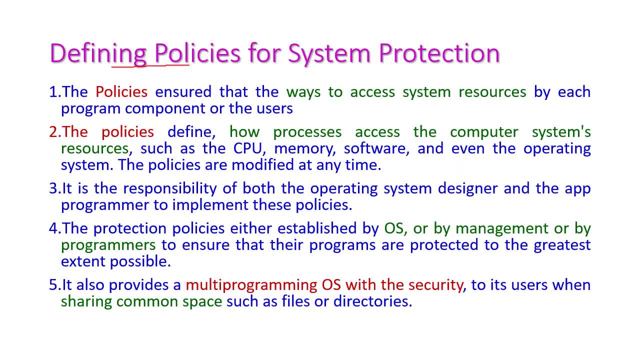 The another important one is defining policies for system protection. The first one is the policy should ensure the ways to access the system resources by the process or by the user. In what way the system resources should be accessed by the other process or other user. 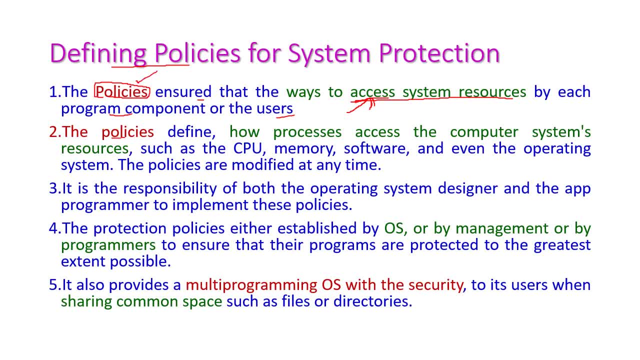 That should be defined in the policy And the policy should define how the process access the computer system resource, such as CPU, memory software and even the operating system, How to access these resources. That should be defined And the policies may modify at any time. 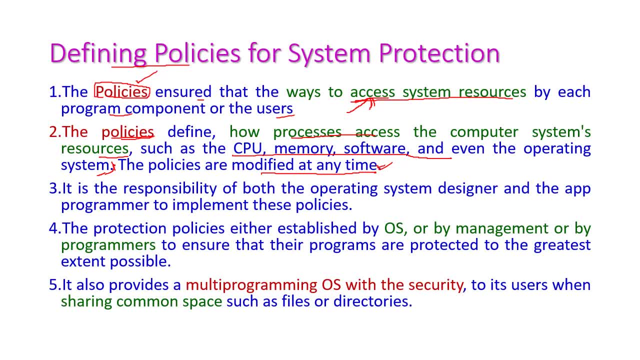 And when come to third one, it is responsibility for both the operating system designer and the application program designer to implement these policies. Who will implement policy? The OS designer or the program designer? And the fourth one, the protection policies. These policies either established by the operating system or by the management, or by the programmer, to ensure that their programs are protected to greatest extent possible. 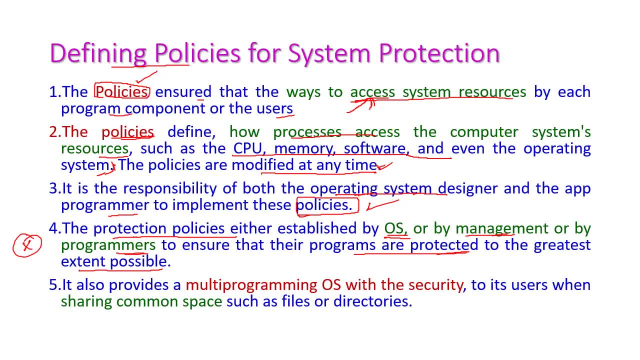 This is another important one, And it also provide multi-programming operating system with the security to its users when sharing a common namespace, Such as files or directories, So the user should feel secured while accessing our particular system. These are the ways to defining the policies for system protection. 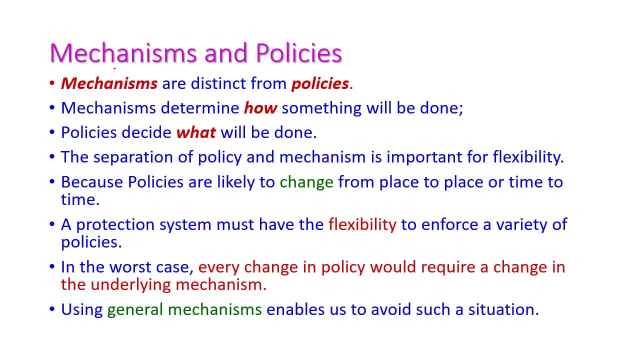 The another important thing is the difference between mechanism and policies, Because mechanisms and policies both are different. Mechanism defines how something will be done And policy define what will be done. These are the main difference between mechanism and policy, So it is important to separate policies and mechanism. 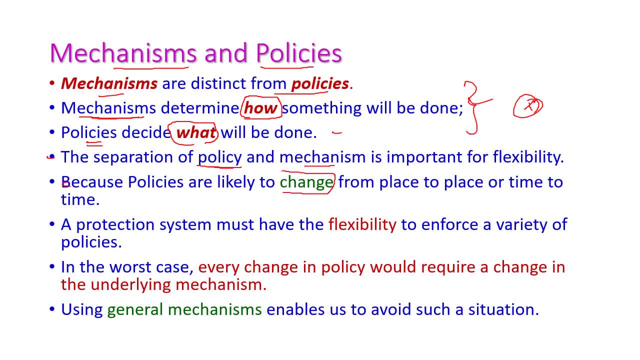 Because policies may change time to time and place to place, But mechanism will not change. So protecting the system must have the flexibility to ensure variety of policies. In the worst case, every changes in policy would require changes in underlying policy. This is the most important thing. 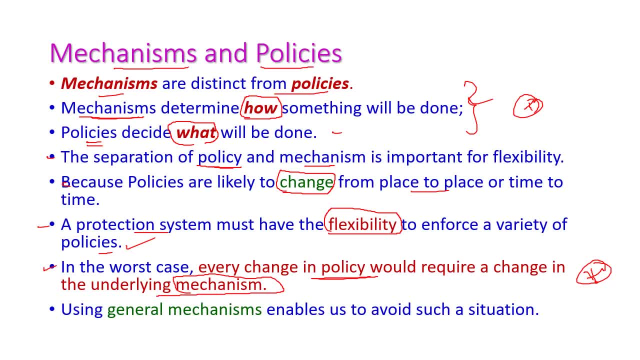 So that we need to separate the mechanism from the policies. So the general mechanism usage will enable us to avoid such a situation. Implementing the general mechanism for designing any system that will be very much flexible for undertaking any type of policies. So these are the main points. 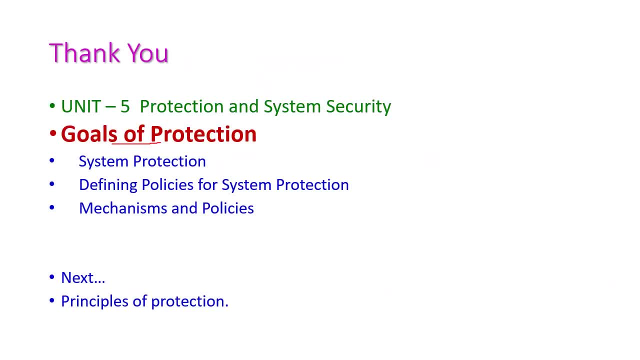 So these are goals of protection. In this class we have defined system protection and importance of system protection And defining policies for system protection and the difference between mechanisms and policies. In next class we will see the principles of protection. 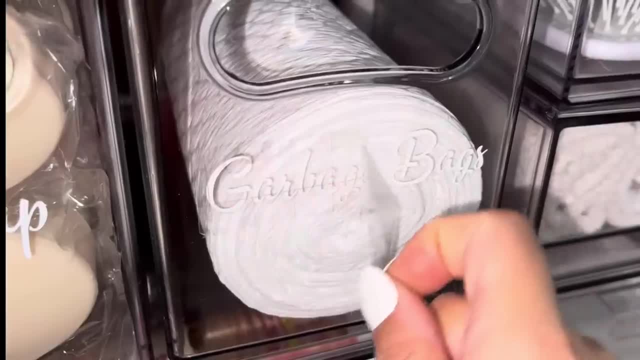 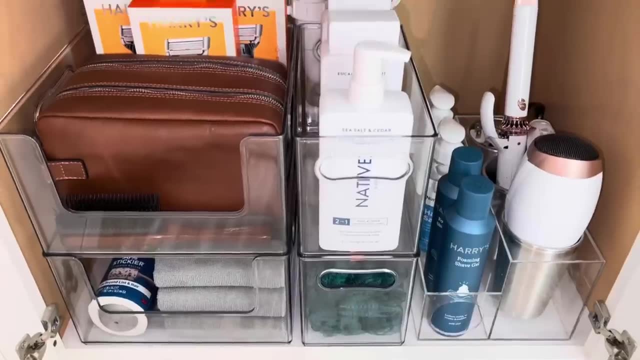 Hey guys, welcome back to Algae Queen Home Decor. I hope you're all having an amazing day. I'm so excited to share this ultimate bathroom organization with you all. If you need ideas, inspiration and motivation to tackle your own bathroom, then this video is for you. 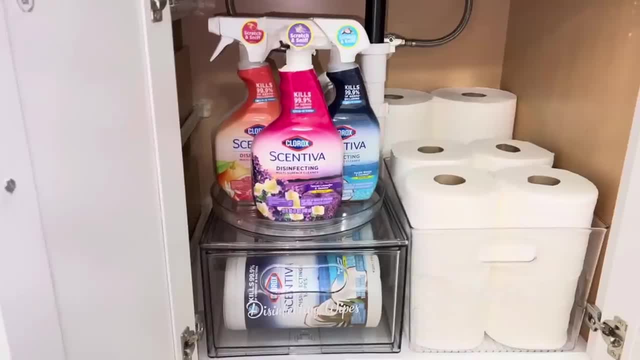 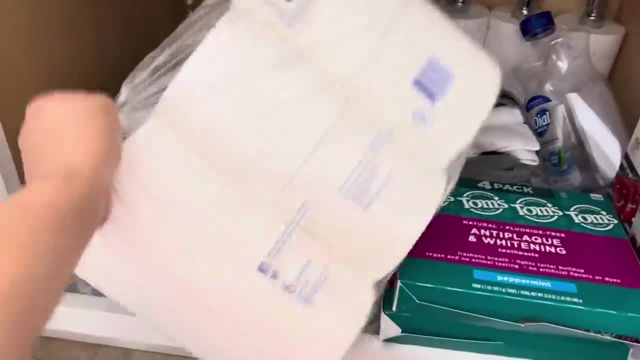 I love taking you all along the process to show you how you can instantly transform any space. I'm so happy with how this bathroom organization turned out on my side of the bathroom, my husband's side and guest bathroom. You will see the before and after: deep cleaning and decluttering to make 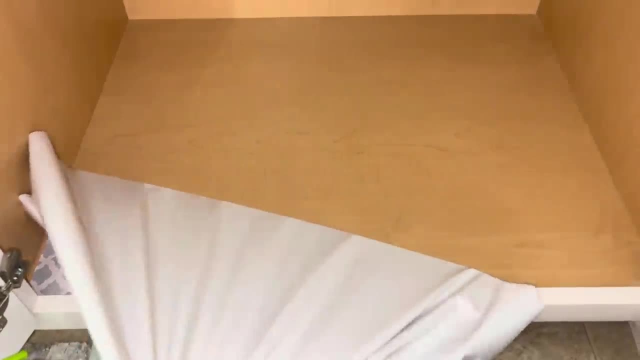 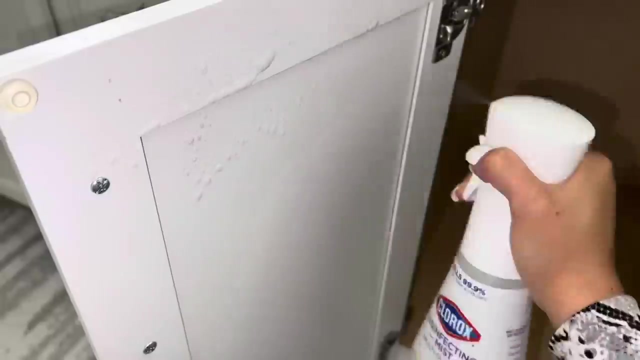 it all more functional and practical for my family and guests. Make sure to give this video a like if you love home organization videos, so I know to keep them coming for you guys Before we continue with the bathroom organization. I wanted to share from being a wife, a parent.